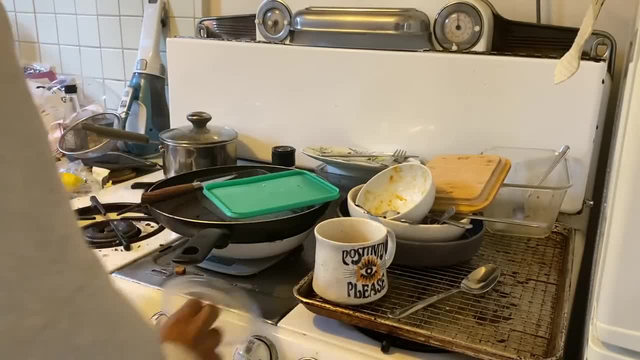 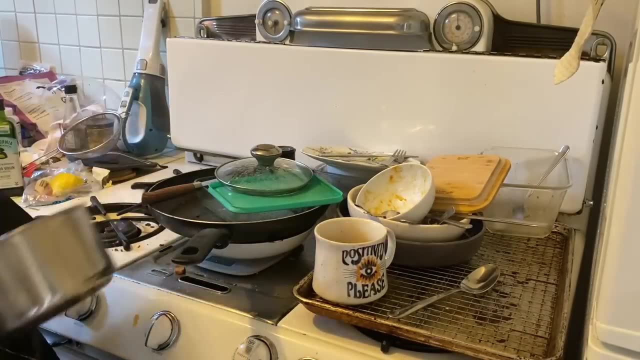 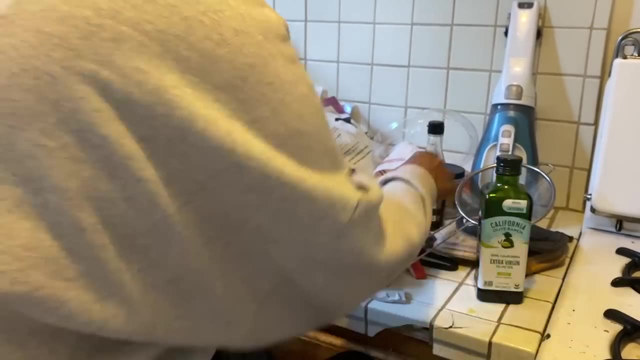 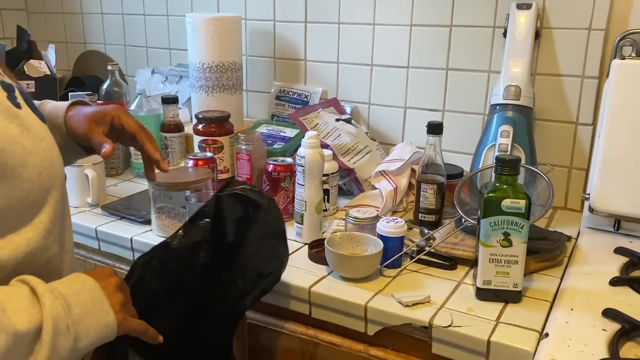 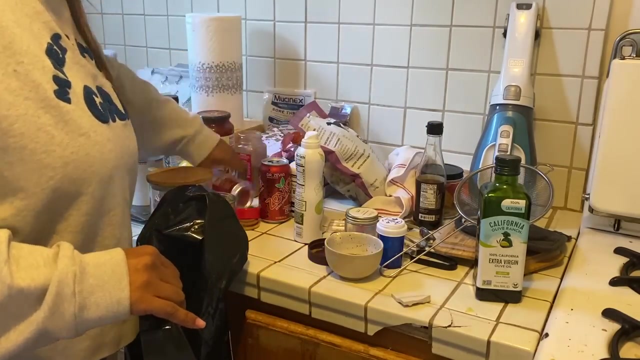 I want to say that decluttering has seriously transformed my life. My house used to look like this 24-7.. Before I decluttered and organized, I always had to declutter. I had to declutter My kitchen in this state Now, I'd say about 80% of the time things are pretty decent in my home. 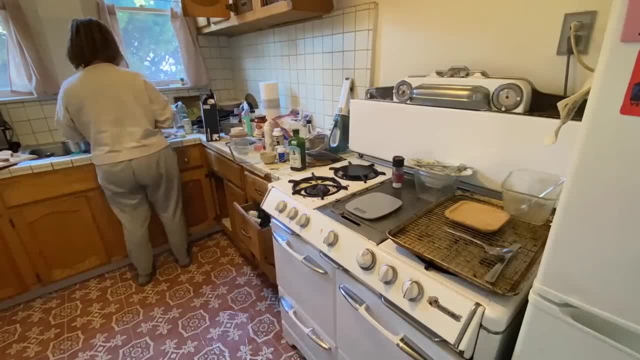 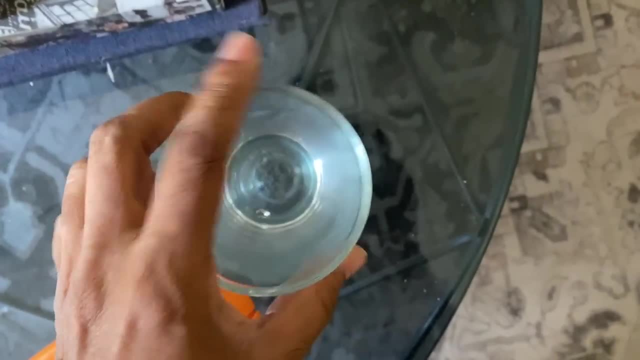 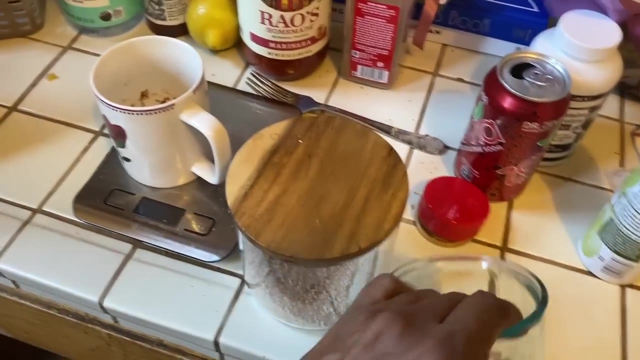 Whereas before it was, 100% of the time, a complete, total hot gangsta mess. It never looked clean, It never was organized, It always had too much stuff. So, yes, I've made a lot of progress. Do I still fall back into old habits and let things pile up? Absolutely I don't know. 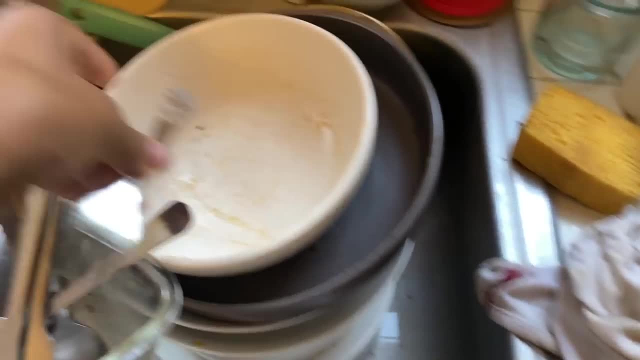 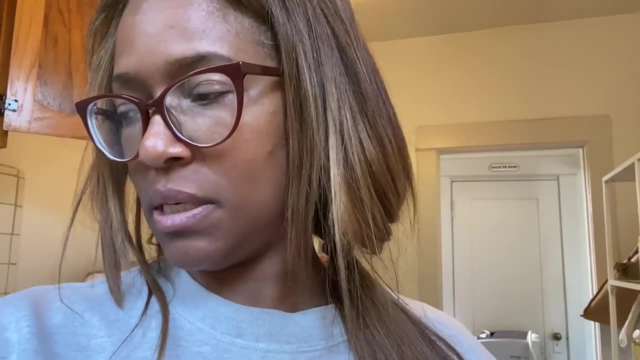 if that'll ever go away. But overall the trajectory is improvement, Progress over perfection. y'all. It's 1235 on the dot. I'm going to see how long it takes me to wash all of the dishes. Let's go. The other thing I'll. 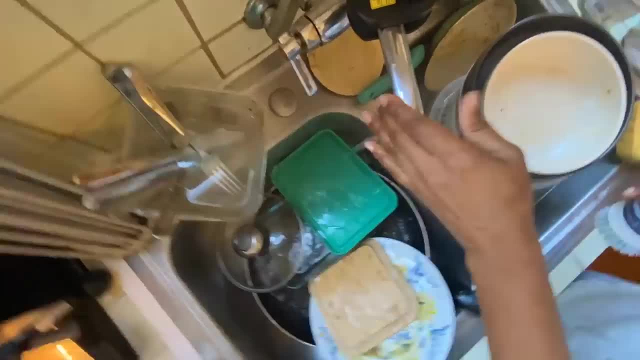 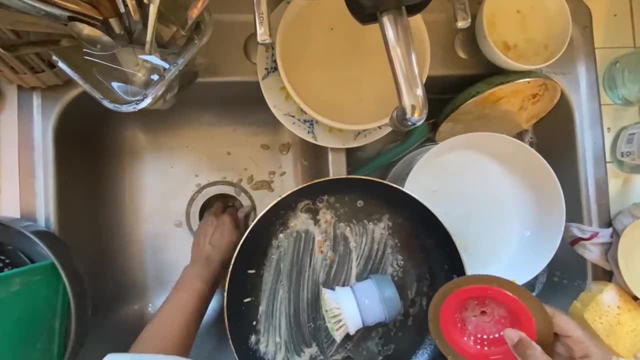 say, is I really love decluttering and organizing and keeping my space more minimal. What I don't love is cleaning. That is something I've learned. I don't like scrubbing floors. I don't like vacuuming, sweeping, doing dishes. 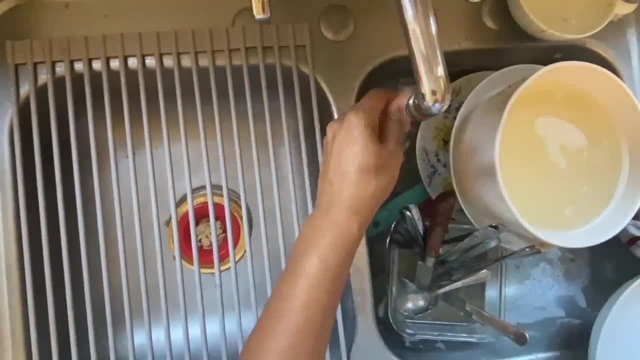 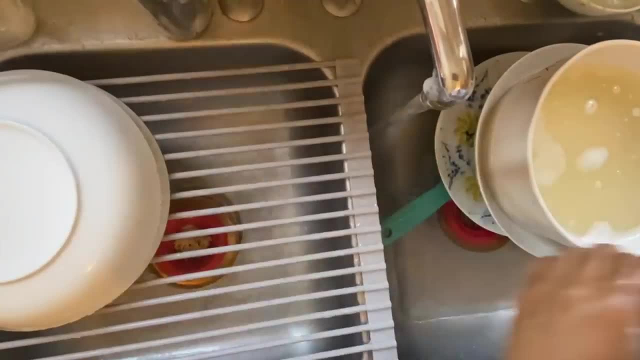 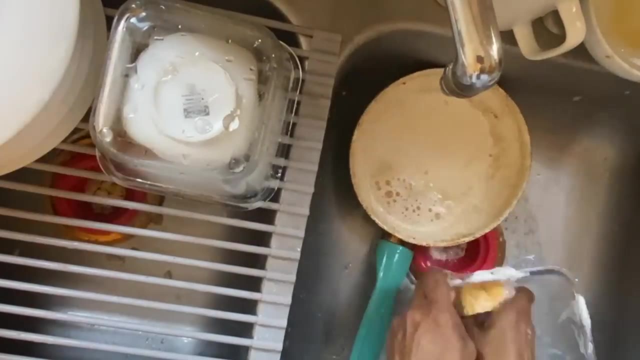 Scrubbing countertops. I don't like it And I really want to hire someone to do these things. I know I'm going to have to do dishes That I'm going to have to do for the rest of my life, Even if I have a dishwasher like loading- unloading, So I've made peace with that. But overall cleaning it's not my favorite thing And I don't think there's any shame in wanting to hire that task out, And it is a goal I have for myself in the new year. 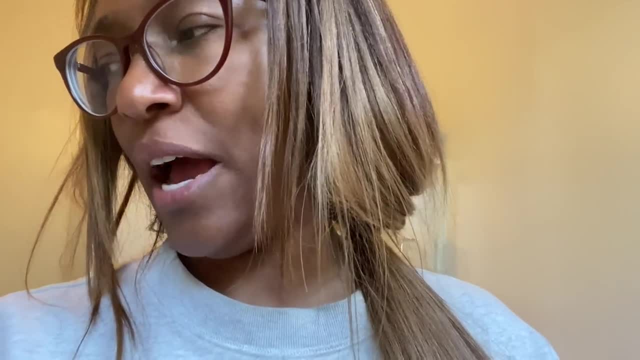 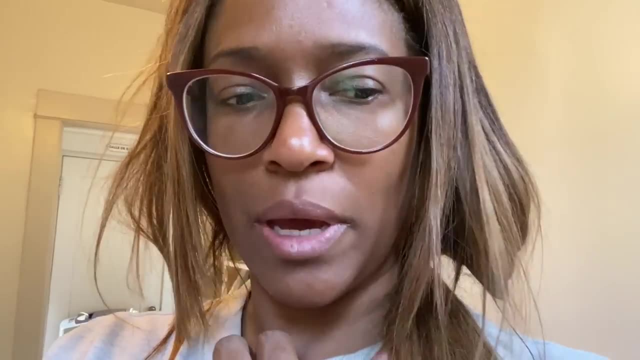 Dishes are done. Okay, that took about 22 minutes, And now I'm going to wipe down the countertops. I'm going to put everything back into its home. So yeah, trash gathered, dishes done, And now I'm going to relocate items that are in the wrong place. 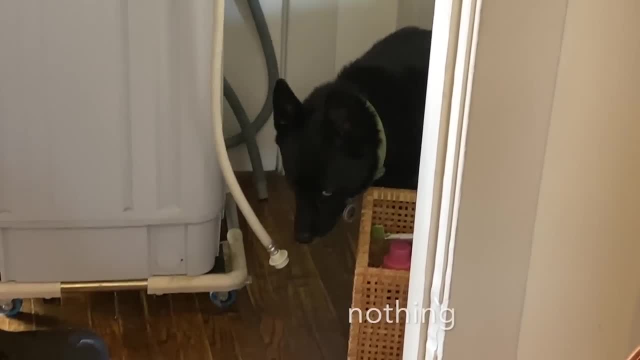 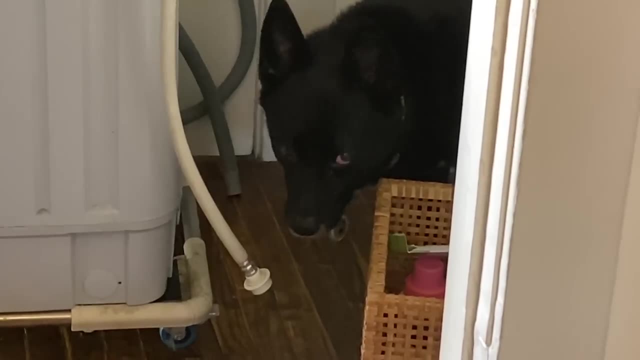 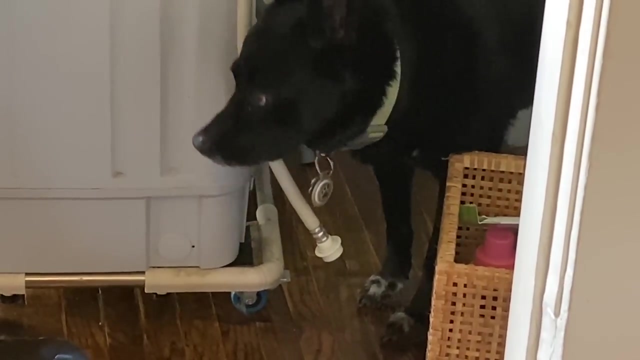 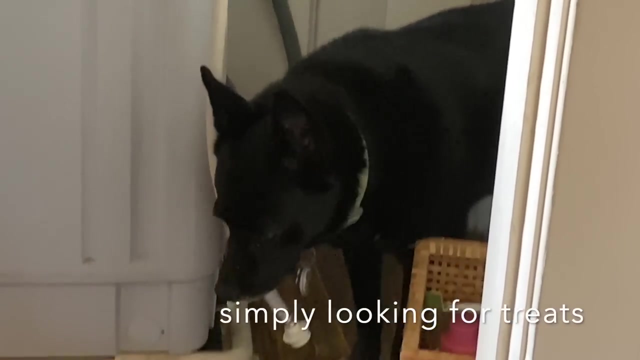 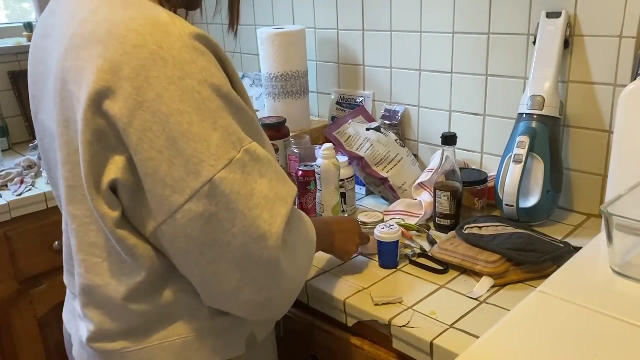 Whatcha doing? You look suspicious. Don't be suspicious, Don't be suspicious. What are you doing, weirdo? All right, all right, all right. The secret to not getting overwhelmed is to just do one item at a time. 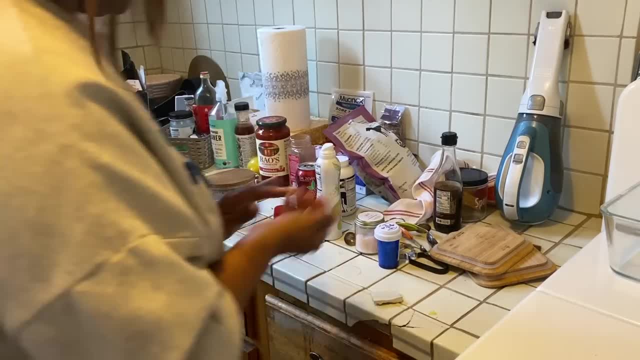 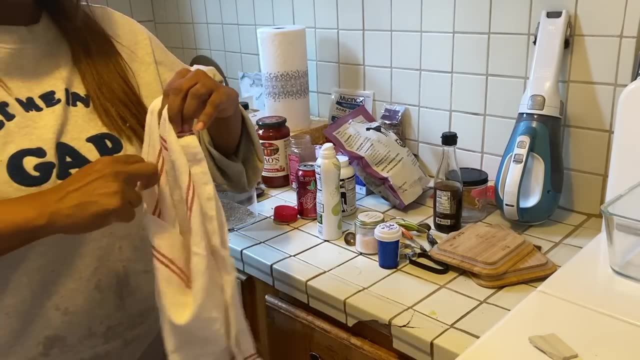 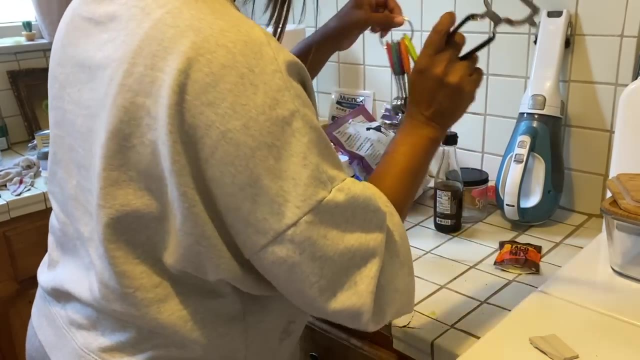 This goes into this bin Trash. This is broken. needs to be repaired. I know where this goes- Same thing. I know where this goes- Same thing, Same place as the pot holder. Lazy Susan Needs to be washed. Lazy Susan. 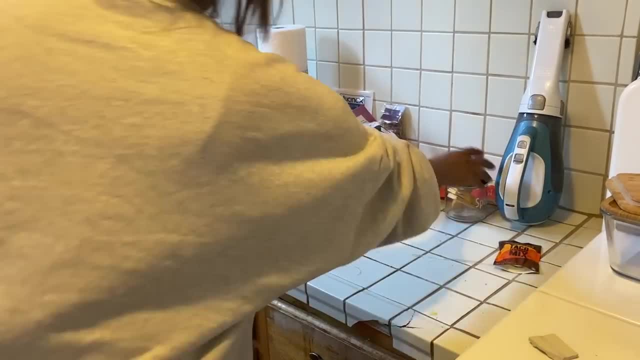 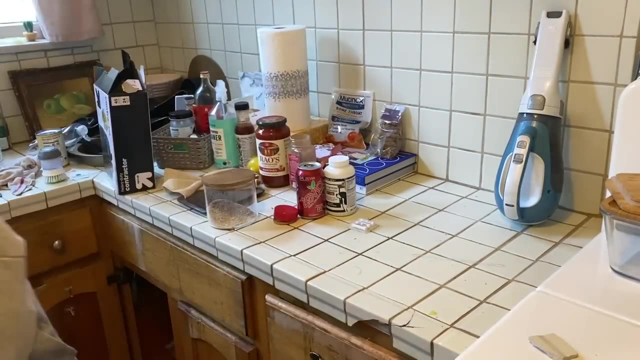 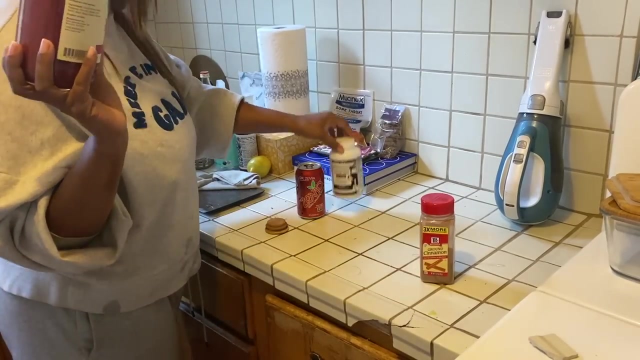 Other Lazy Susan Under the sink. That's why it's great to organize, because then everything starts to have home Samson's bag. It's going to go in the bathroom Upper cabinet. This goes in the pantry cabinet. See how much medicine. 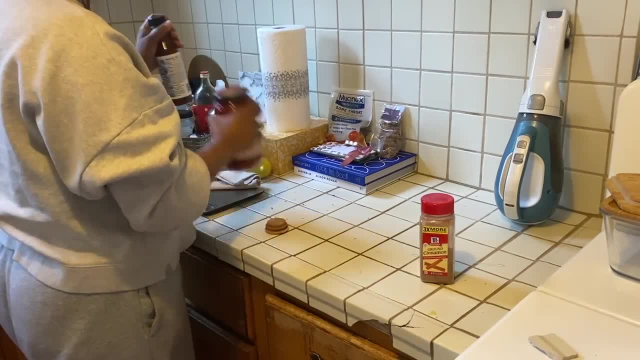 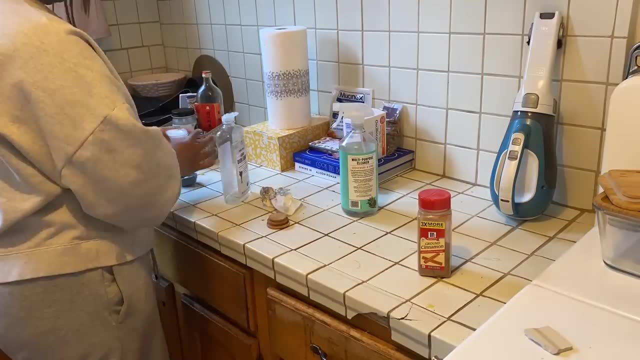 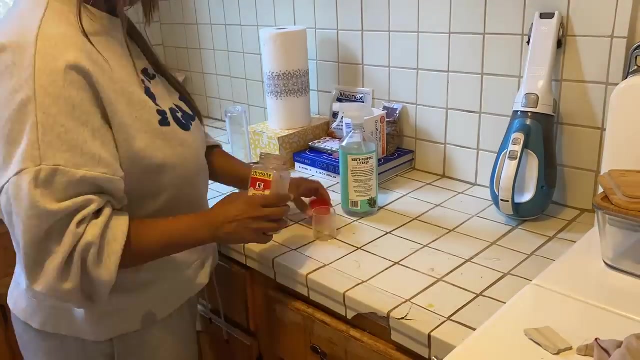 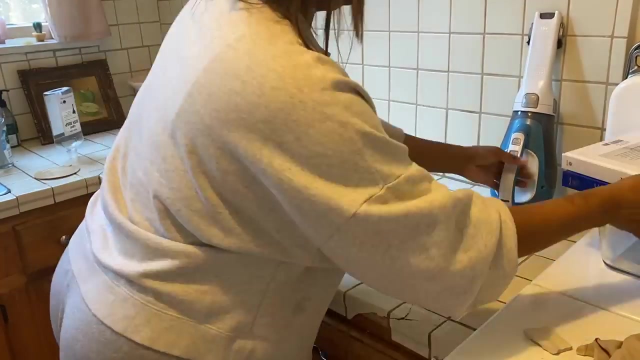 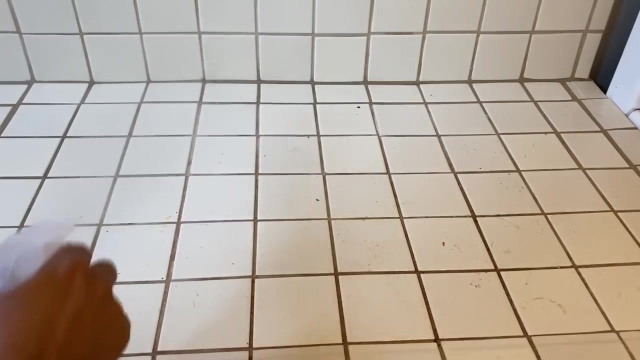 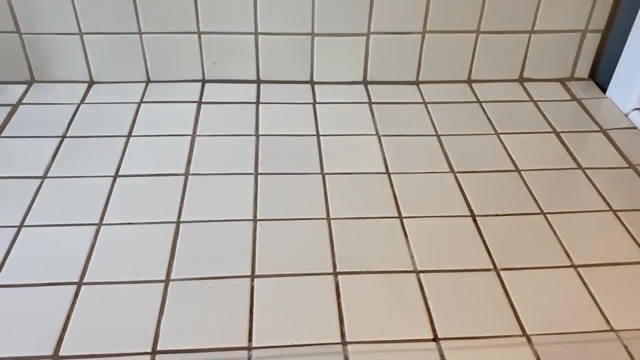 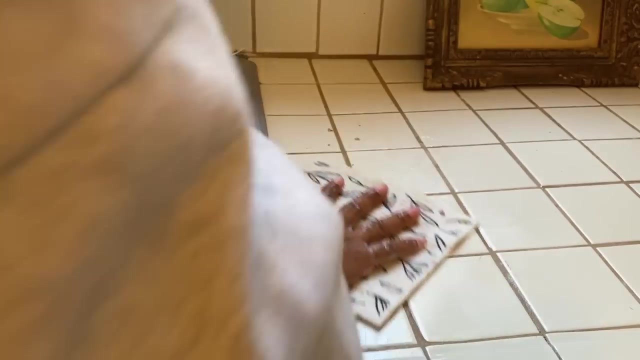 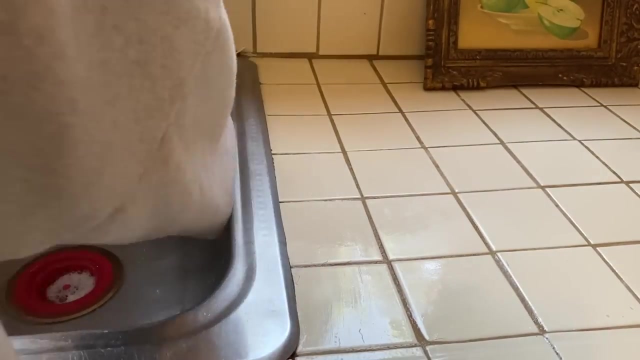 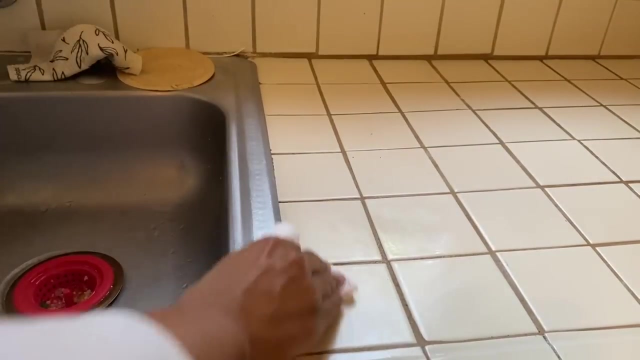 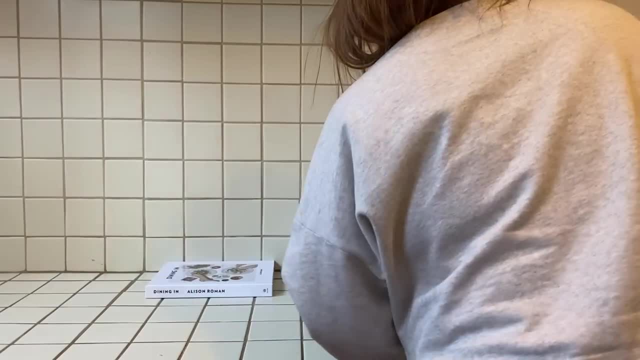 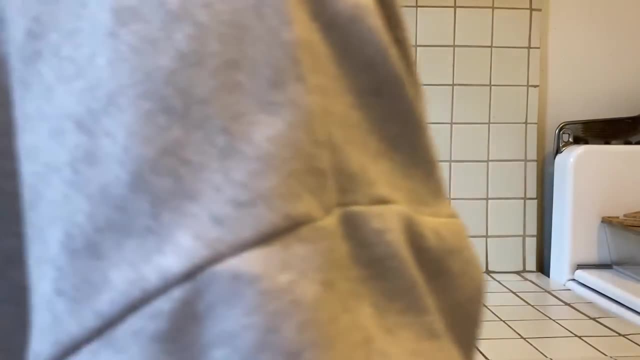 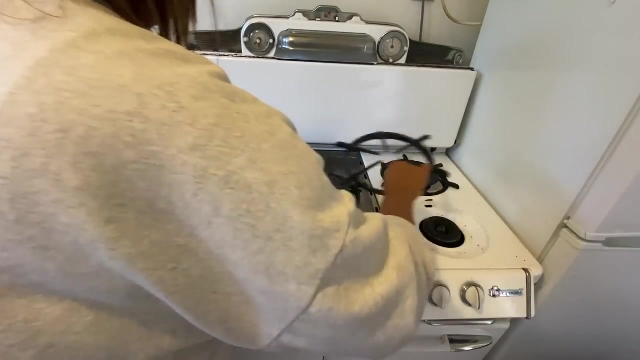 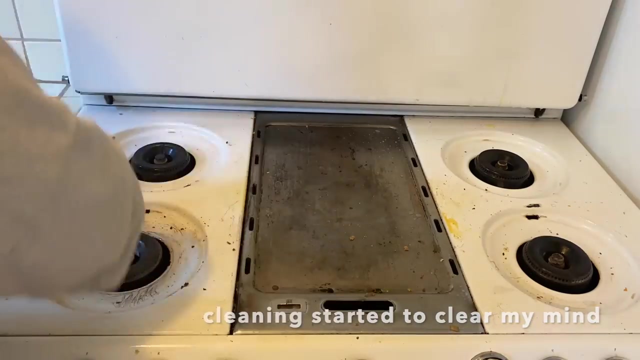 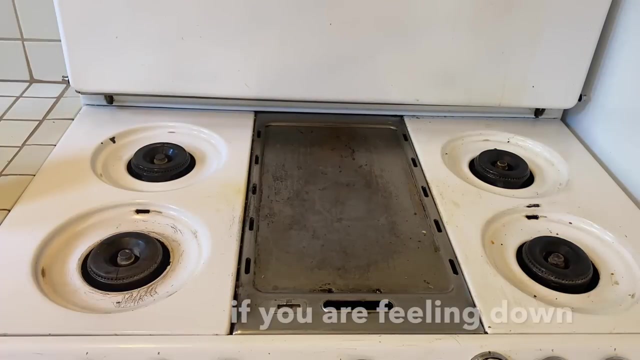 and cook for about 1 hour. when the water boils, turn off the heat and cook for about 5 minutes. I'm going to use this as a tablecloth and I'm going to use it as a tablecloth and I'm going to use it as a tablecloth. 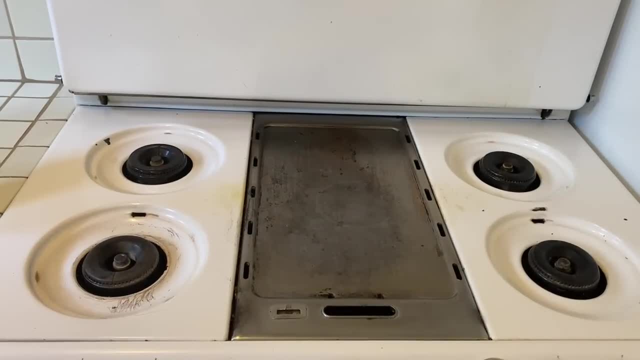 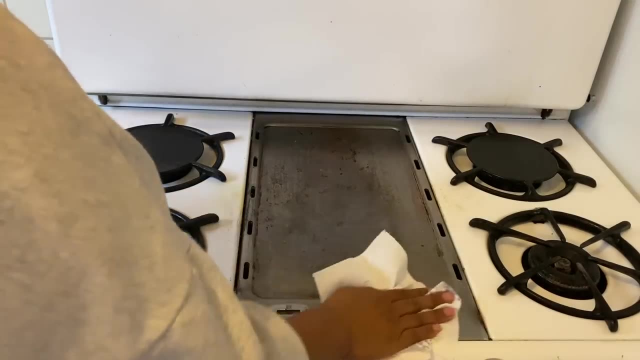 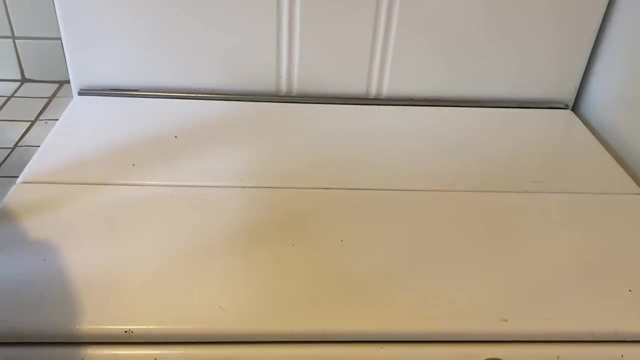 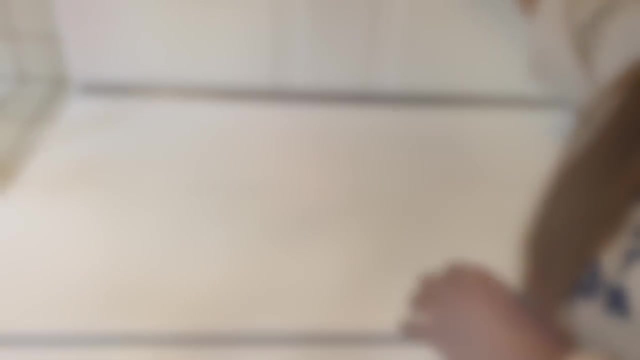 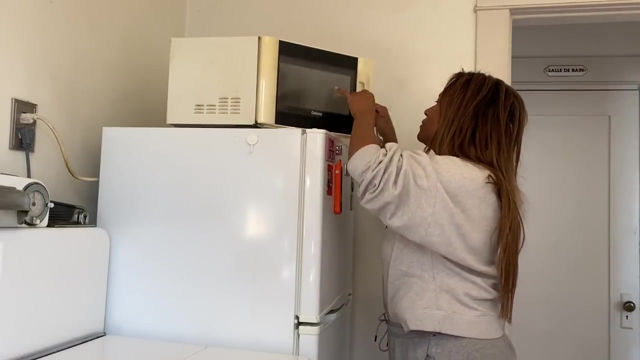 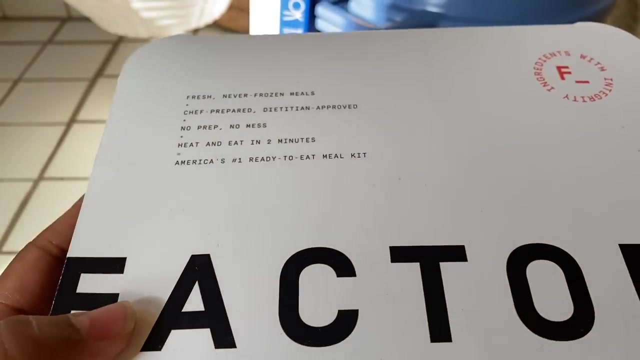 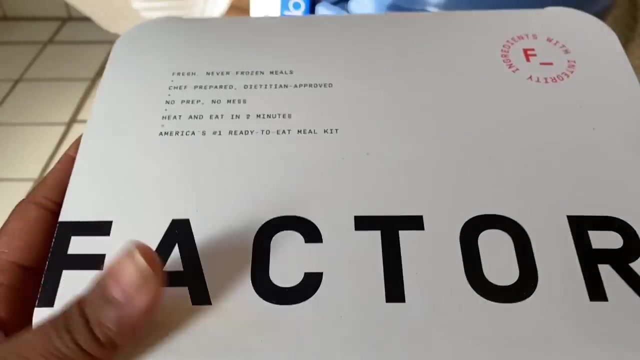 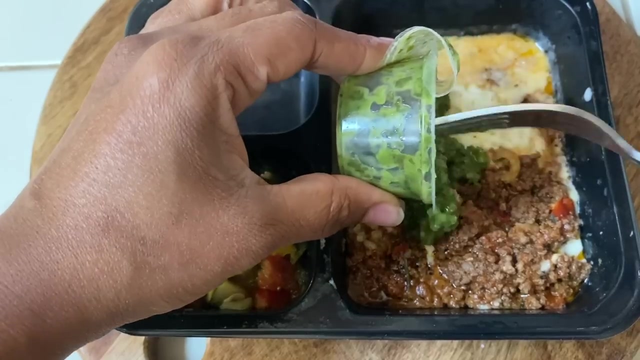 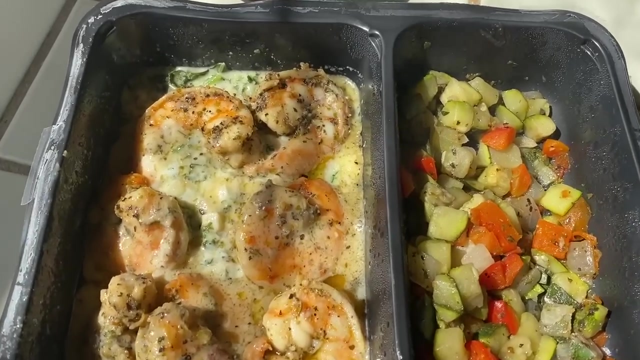 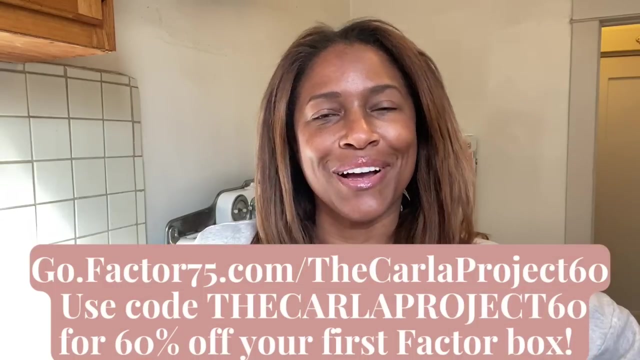 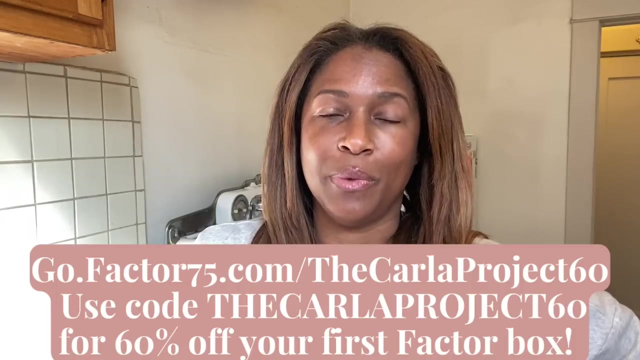 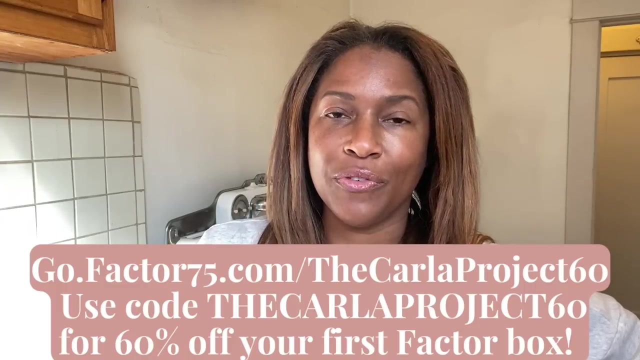 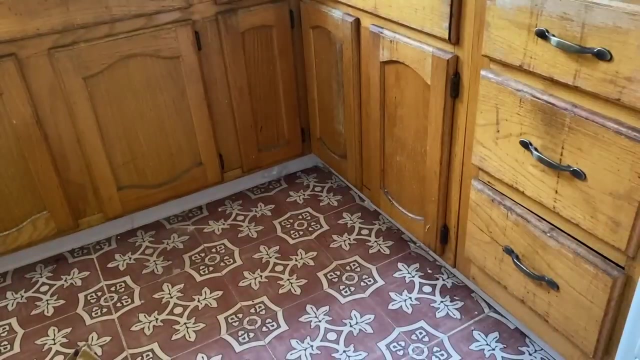 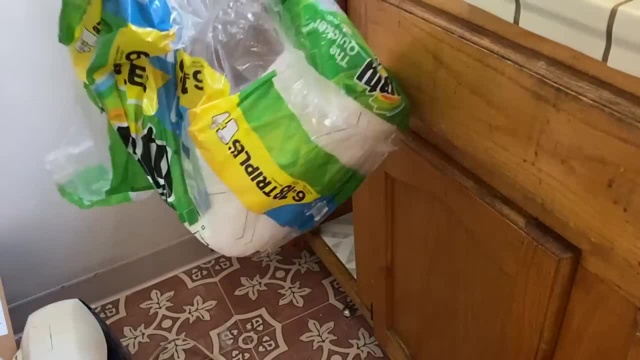 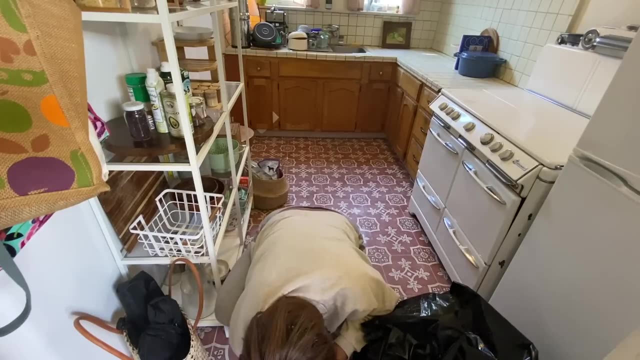 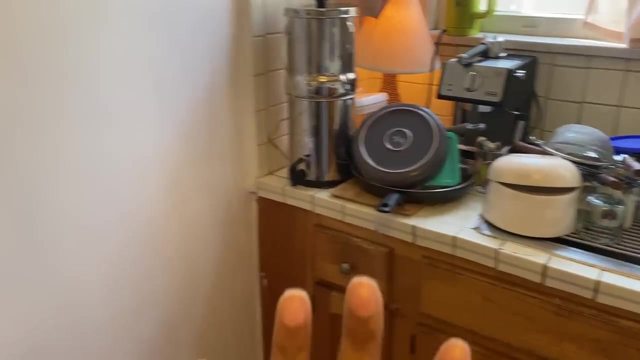 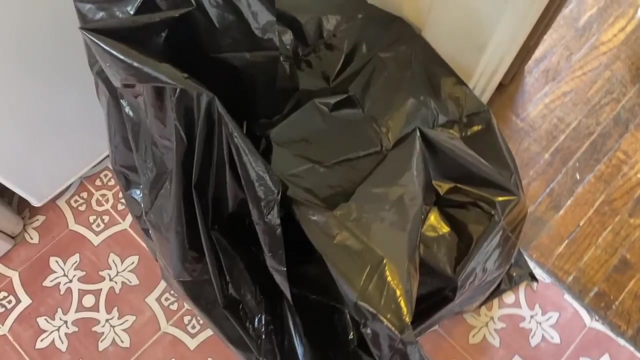 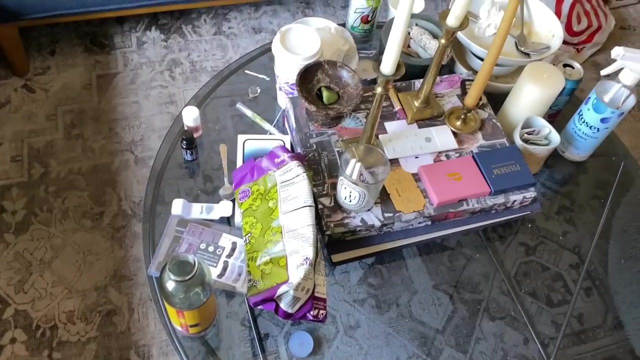 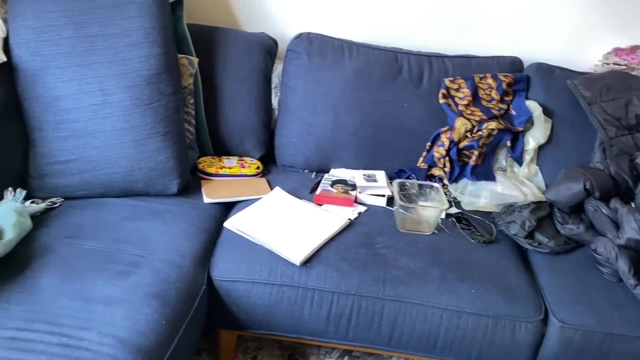 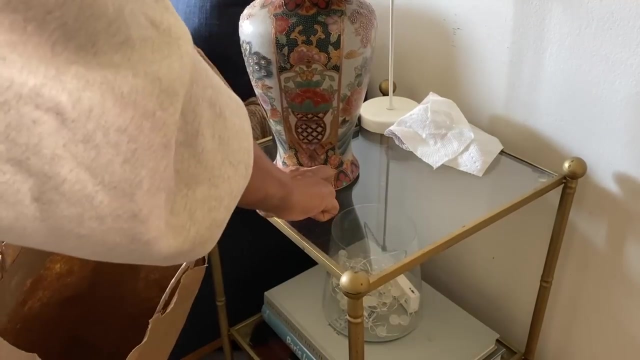 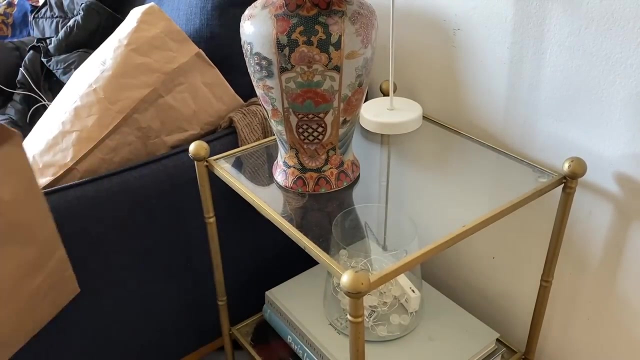 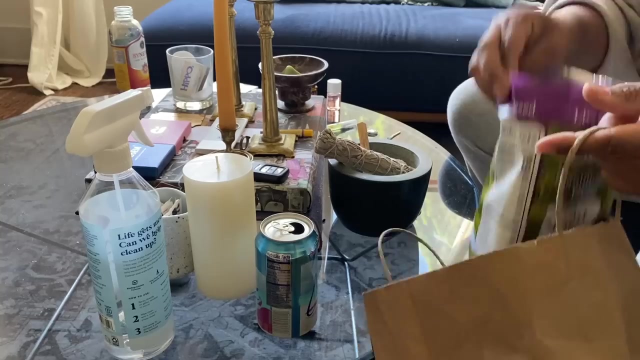 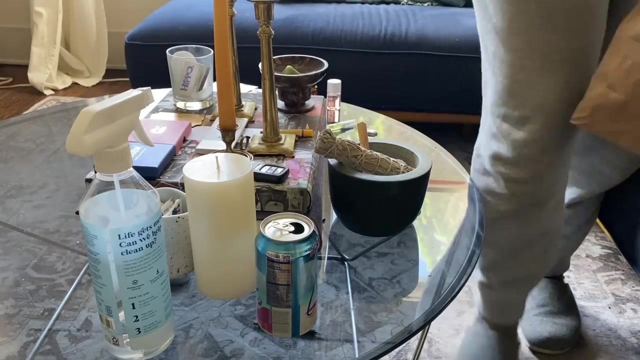 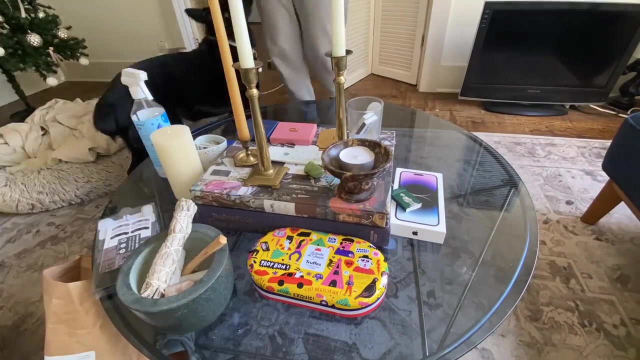 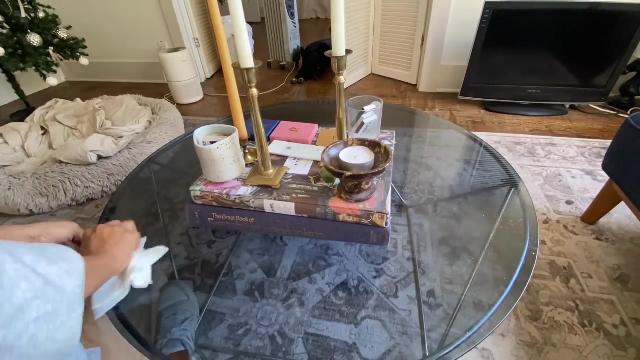 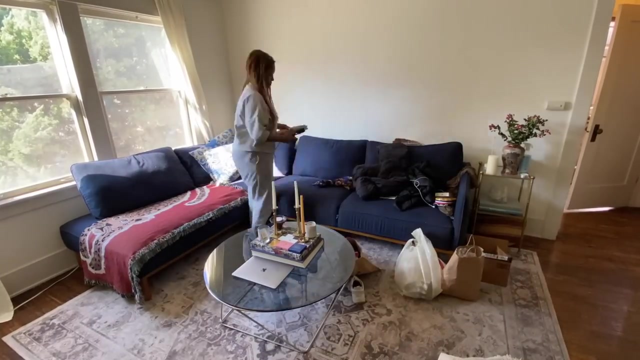 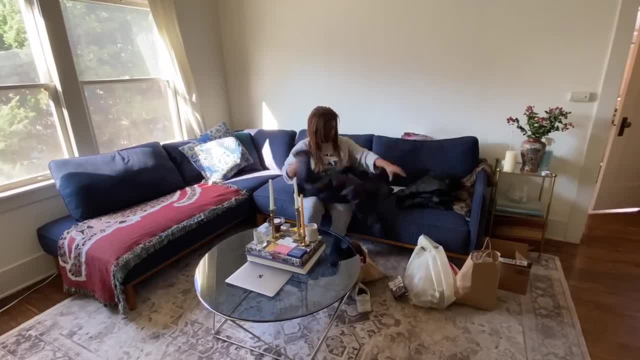 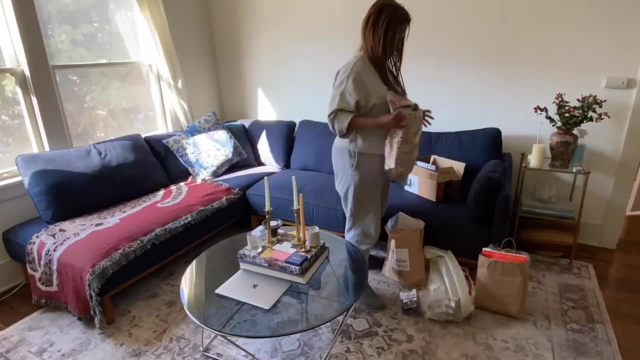 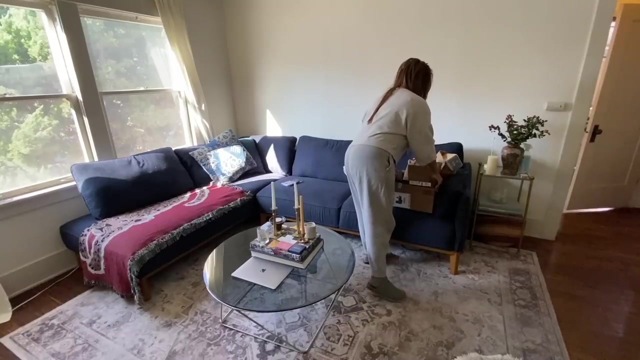 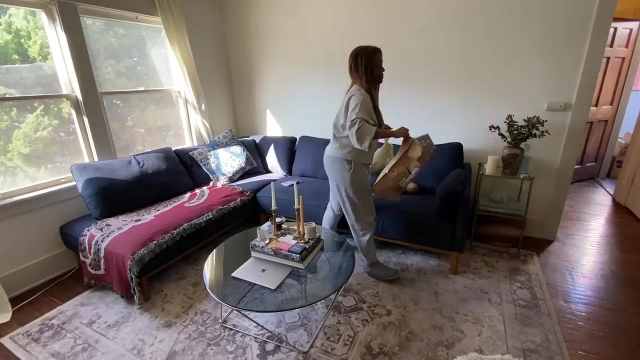 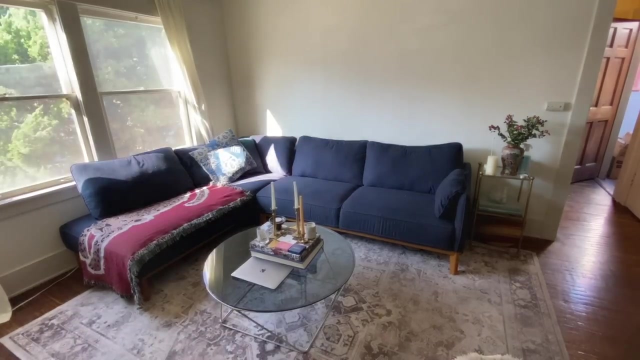 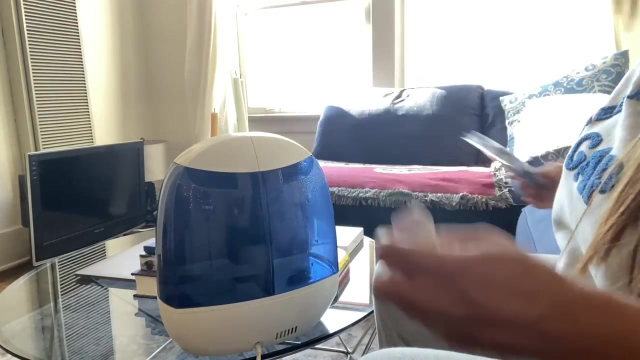 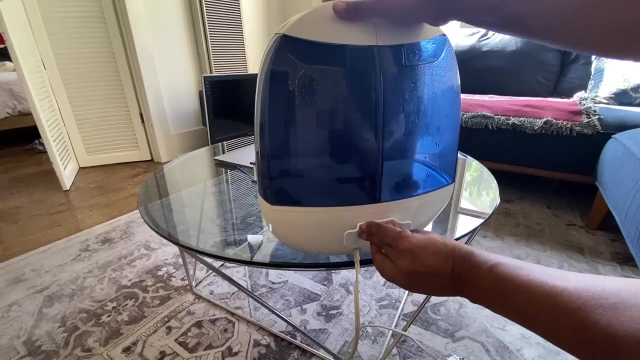 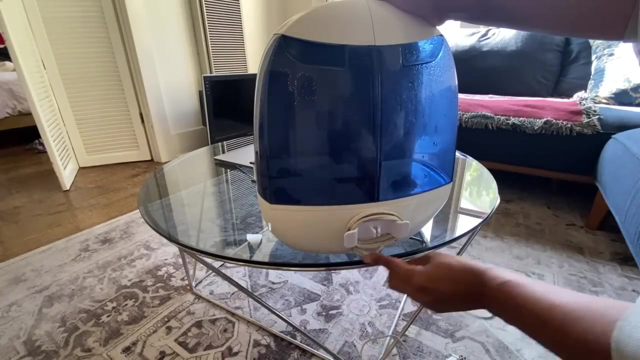 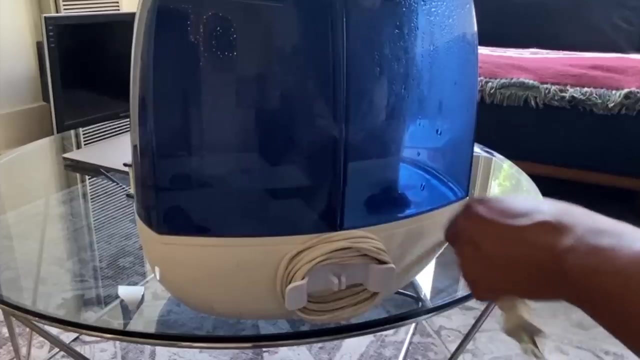 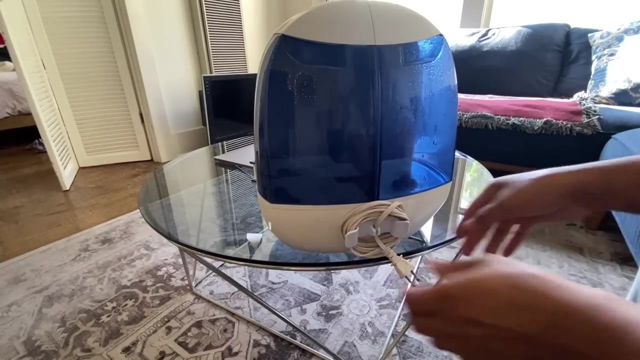 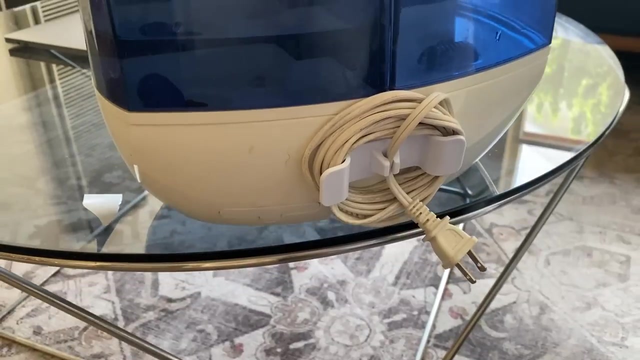 I'm going to use this as a tablecloth and I'm going to use it as a tablecloth. I'm going to use this as a tablecloth- Literally a genius. How cool is that? That's amazing. No more loose cords. I'll link it in the description box. I'm gonna do it for my. 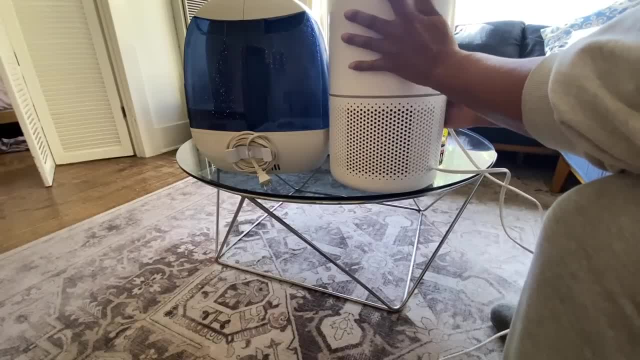 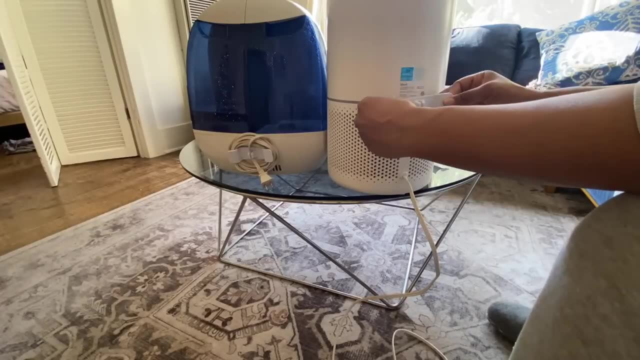 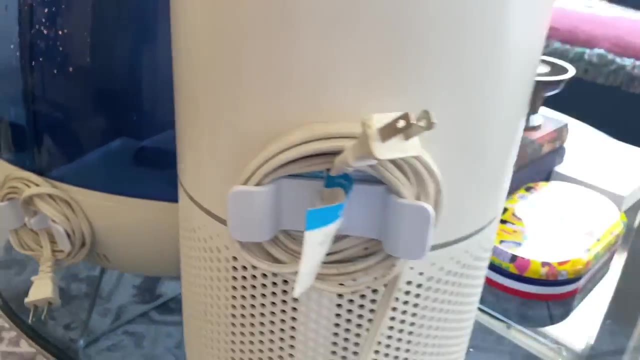 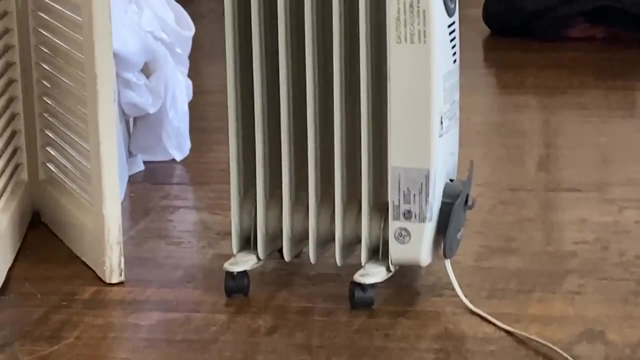 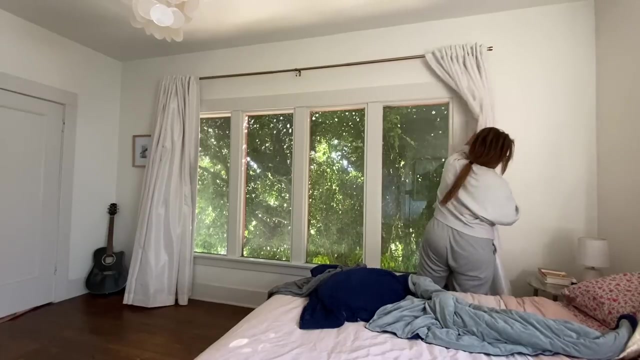 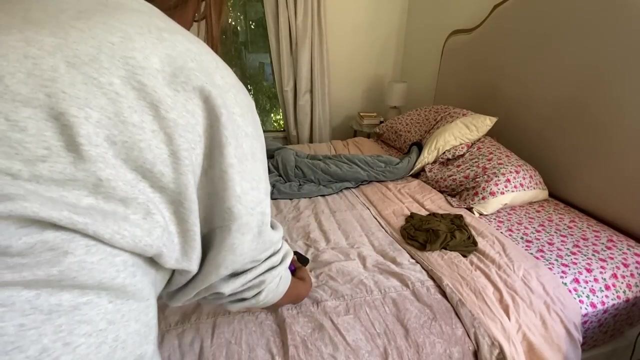 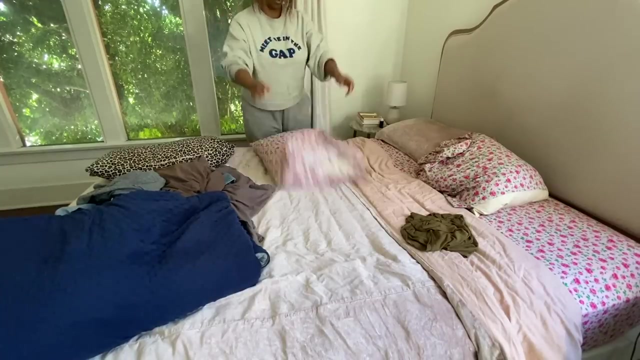 air purifier too. Like all of these should come with cord winder. That's amazing. These would just be loose cords on the floor. That one comes with one. It's broken, but it does have one, So I'll just use it. 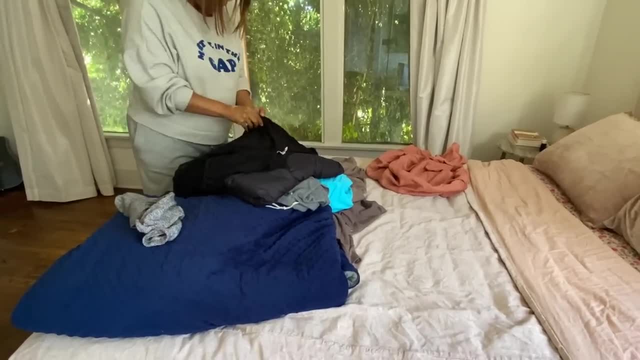 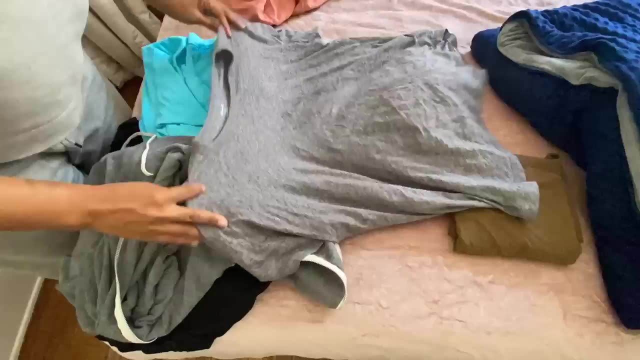 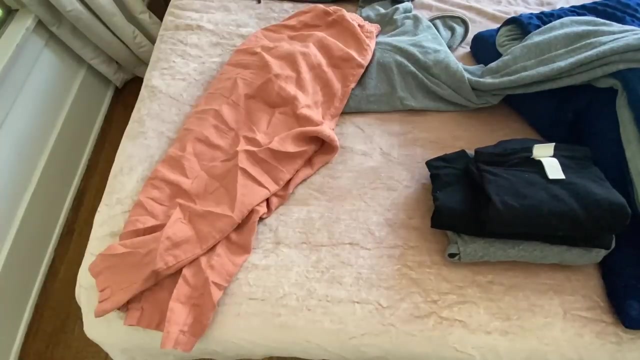 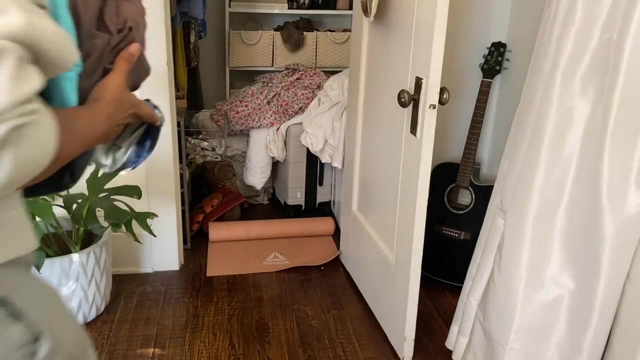 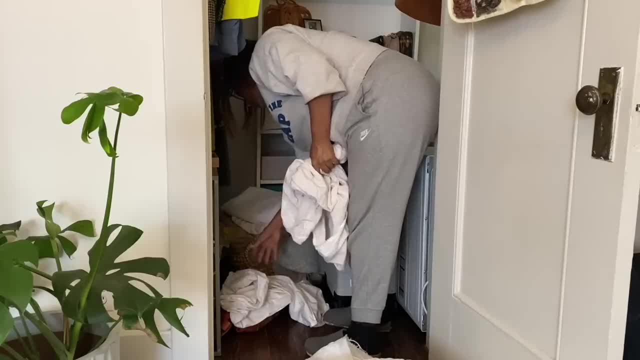 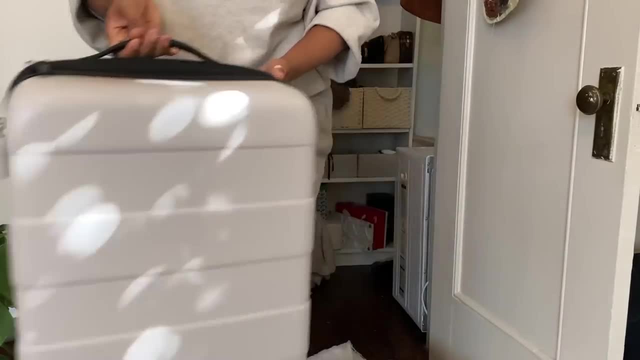 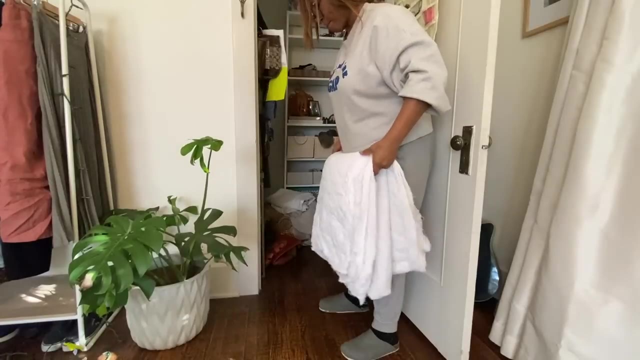 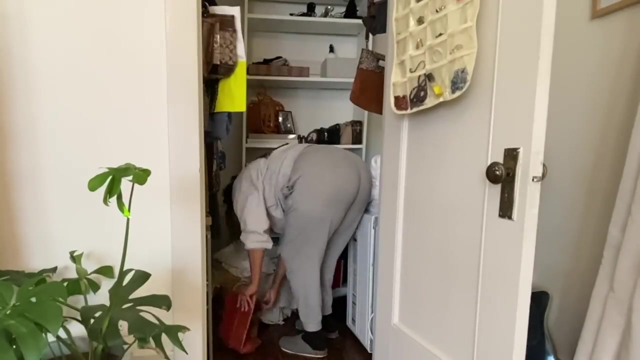 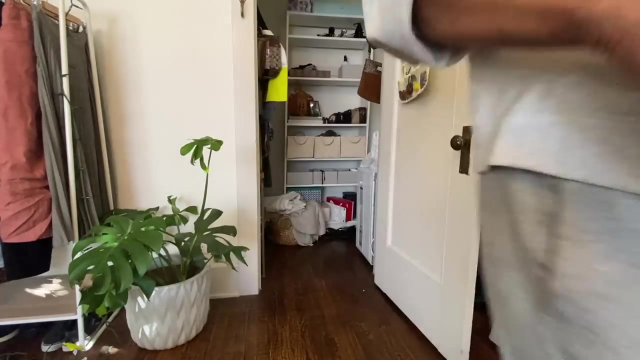 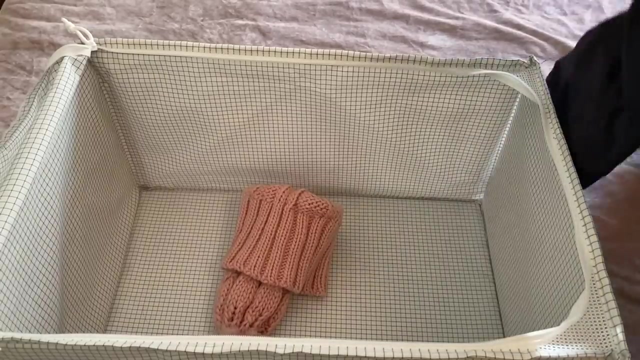 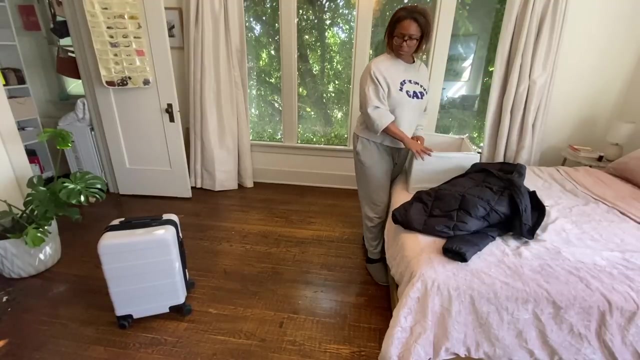 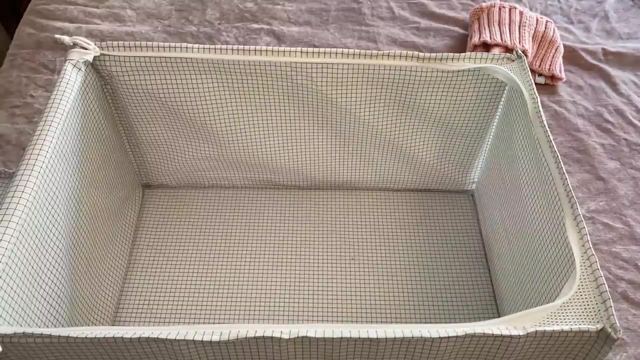 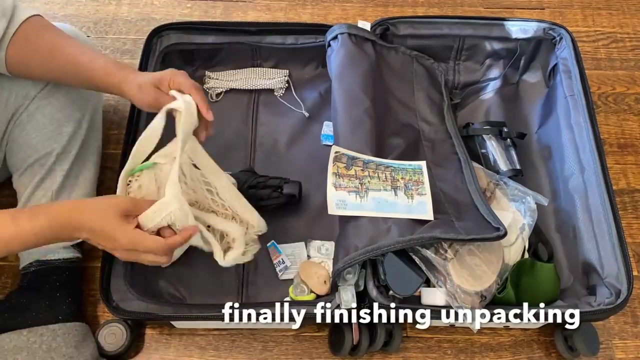 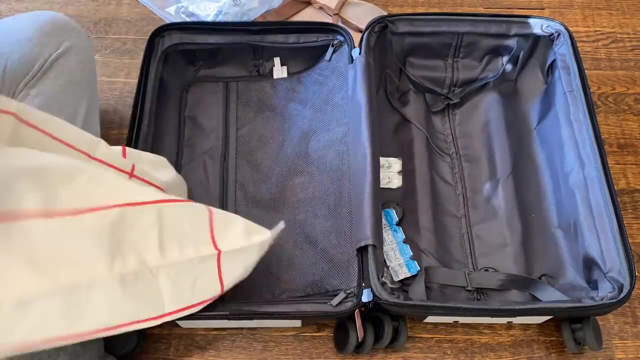 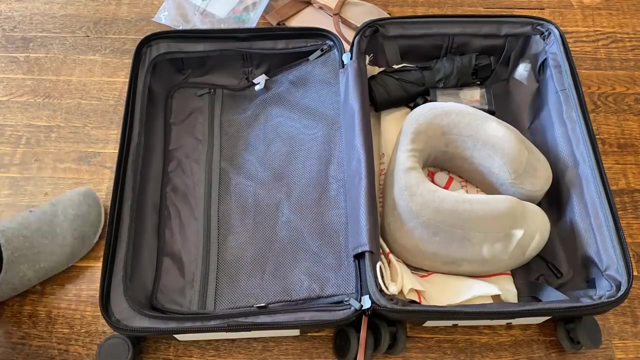 Thank you. This is my seasonal box and I'm going to put the coat that I brought with me on my holiday into this bin. I'm going to take my swimsuit, put it in here and my giant scarf. Okay, here's the random stuff that was left in the suitcase. 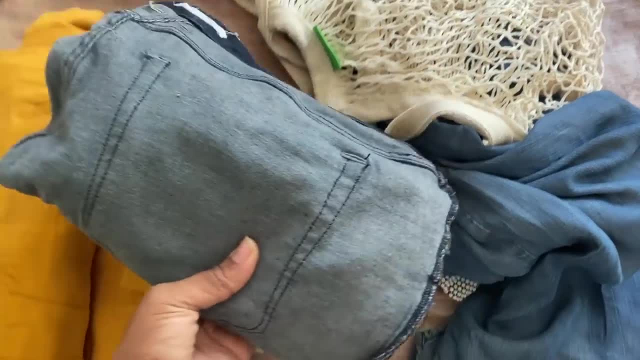 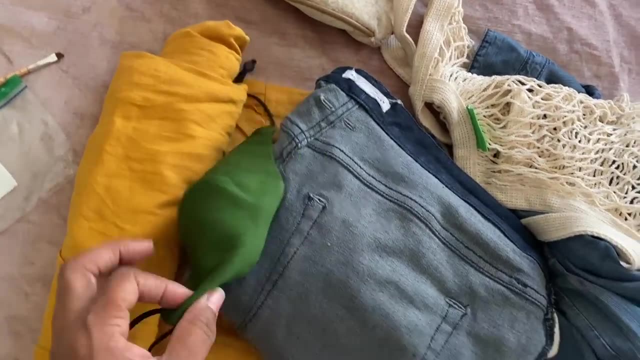 These are the two items I did not wear. All the other clothing I brought with me I wore, So I'm going to hang these up. This will go in the dirty clothes basket. This will go where my masks go. Where's my other one? 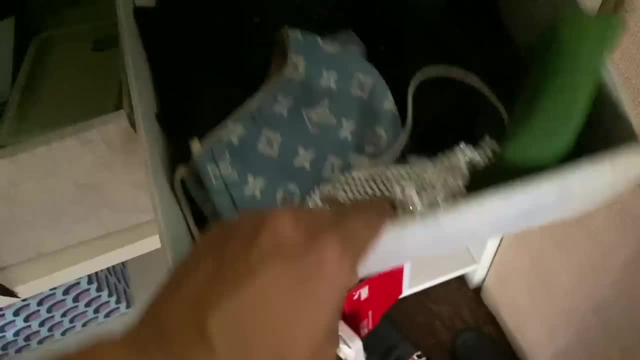 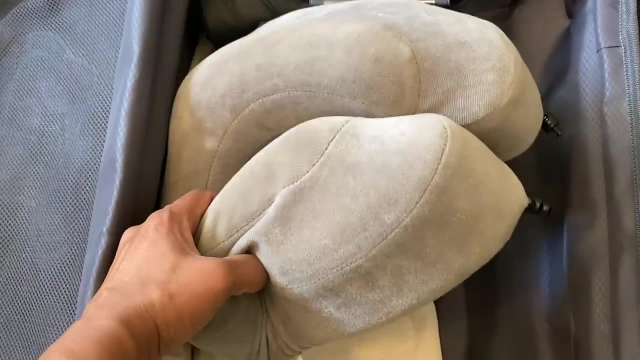 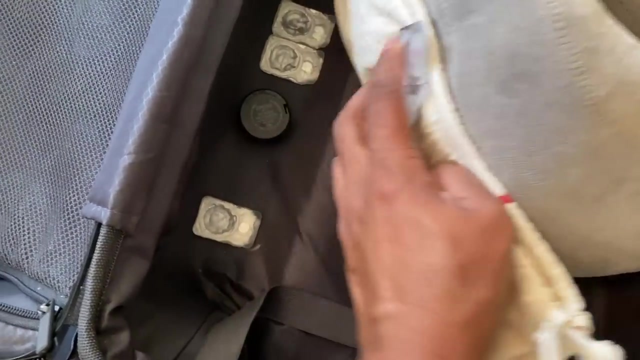 So this belongs in here: My little mask box, And then, for the suitcase, I'm keeping anything travel-related in here: My neck pillow. this bag I use dust bag, I use as a laundry bag. Oh, oops, missed a few things. 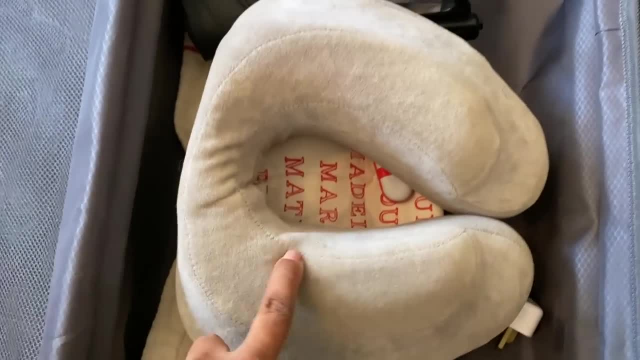 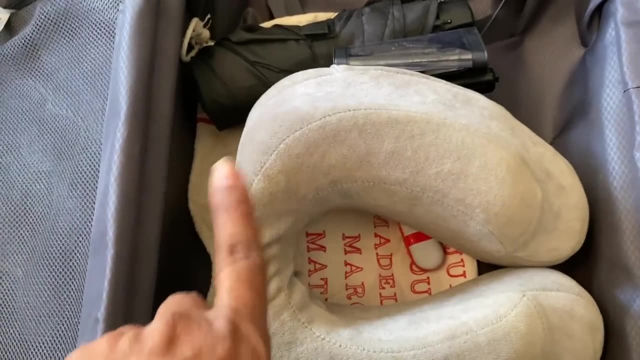 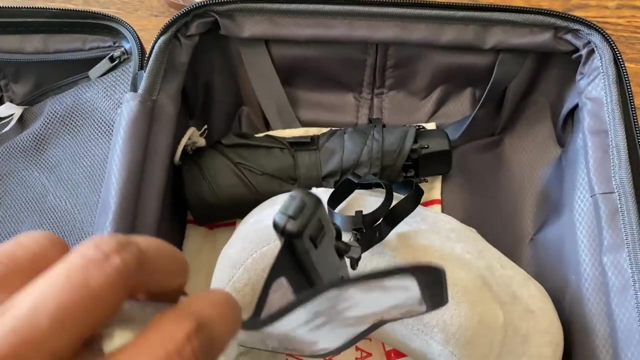 Contacts: my eyeshadow, Airplugs for the plane Travel umbrella travel plug And this I'm on the fence about keeping Underwater phone holder. I don't know. I'm going to keep it in here for now. 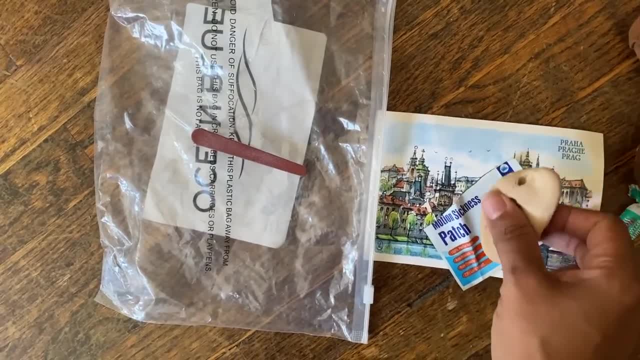 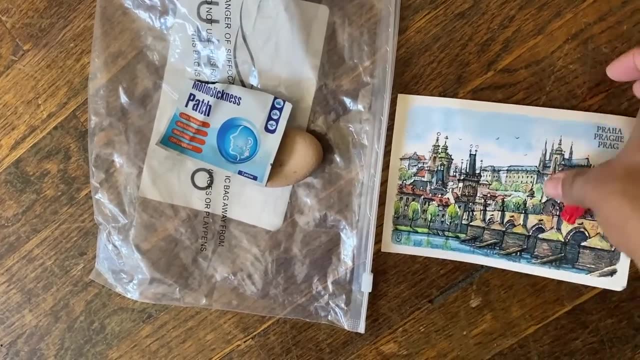 Okay, throwing away this bag, Little nail file, a rock that I got from the beach in Italy. I don't really need that. Okay, Okay, Okay, Okay, Okay, Okay, Oh, my gosh, Oh my gosh. 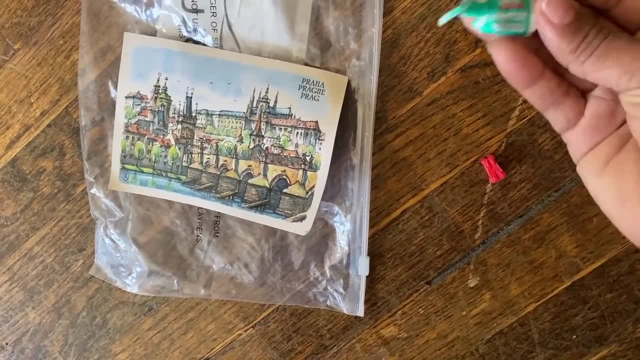 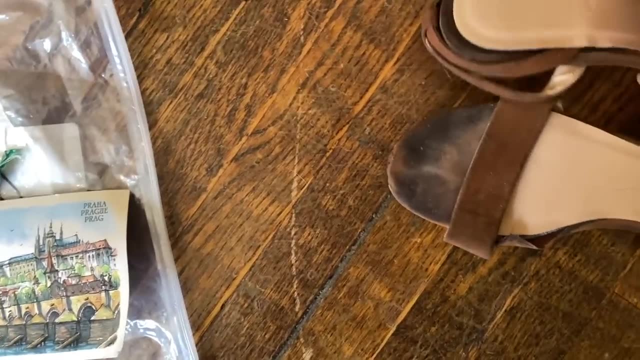 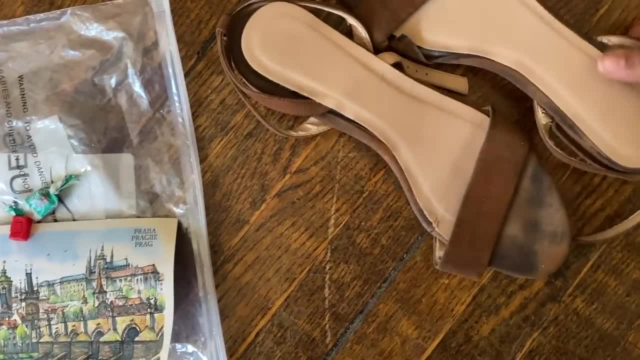 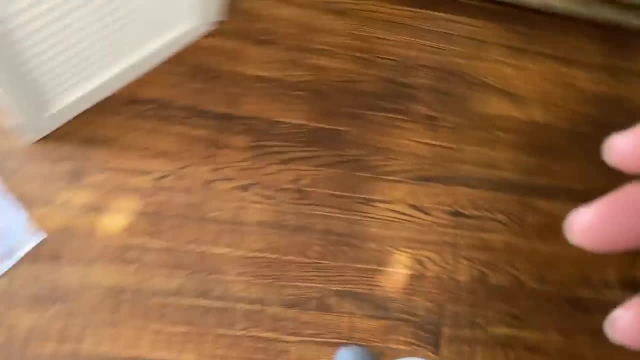 I need to find a replacement. I'll work on that this month, But for now I'm going to keep them over here. Oh my gosh, Oh my gosh. Throw this stuff away. I love this hanging organizer. 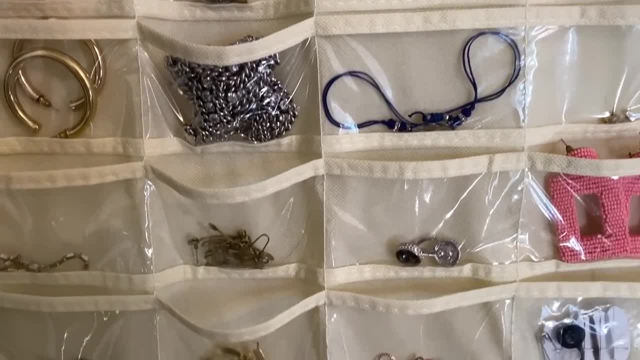 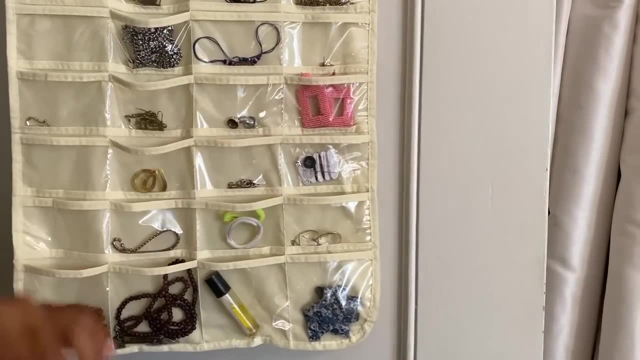 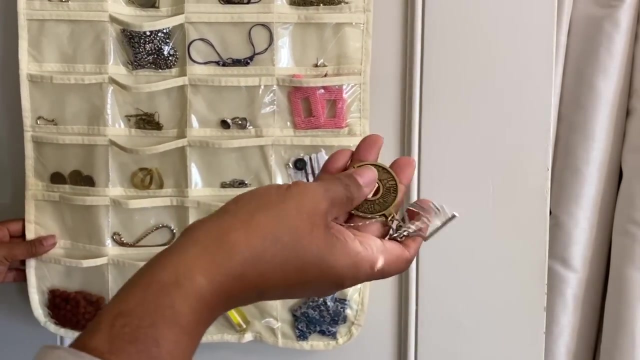 It's really for jewelry, but I've started using it for all kinds of little knickknacks. Some of my hair ties are in here I'm going to put this mini sewing kit, The coins that I got from other countries And this, actually this I'm going to put in the bathroom my biomedic necklace. 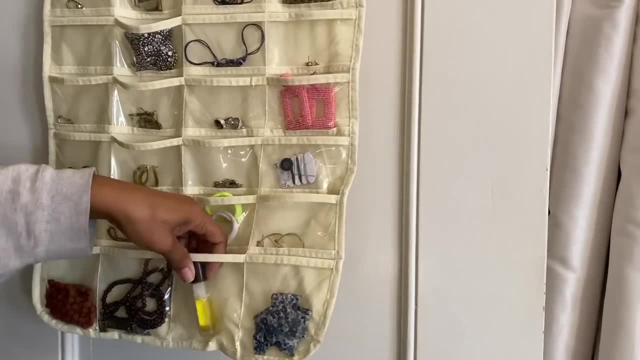 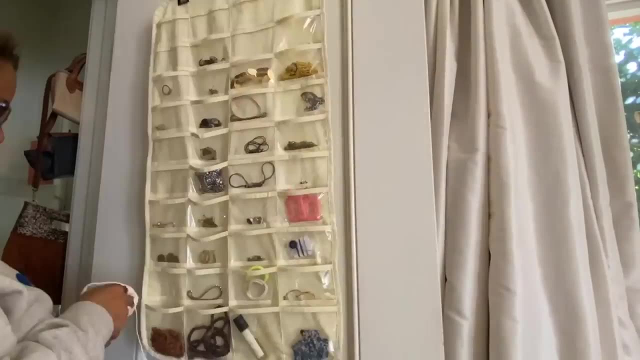 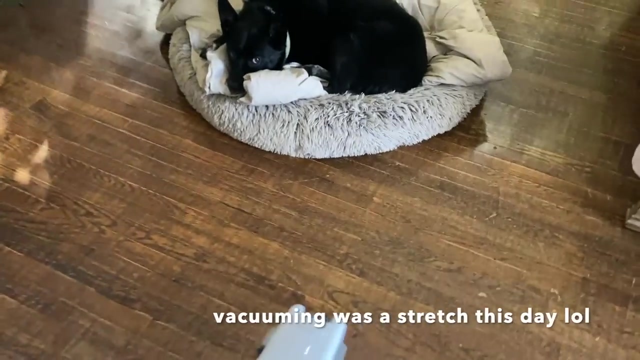 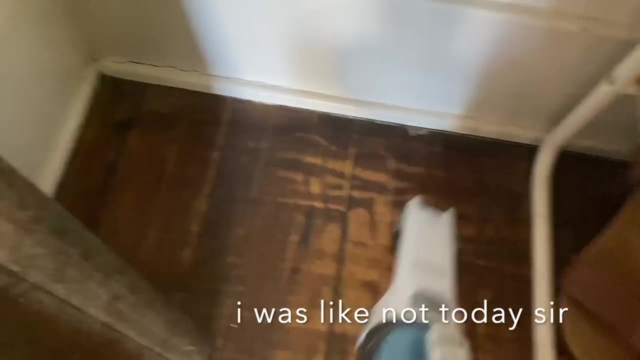 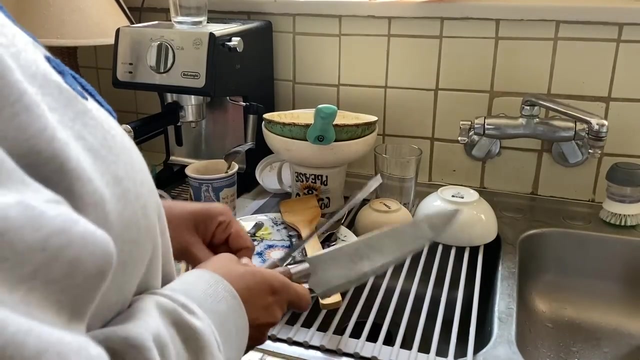 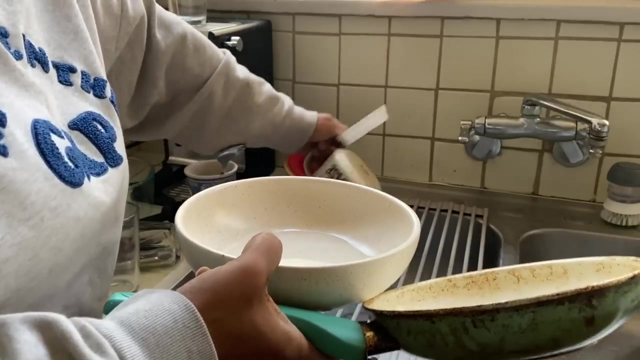 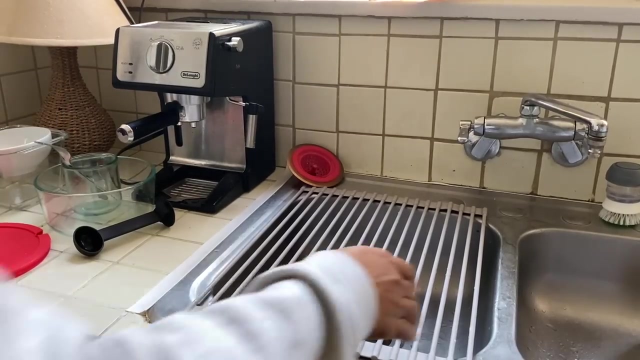 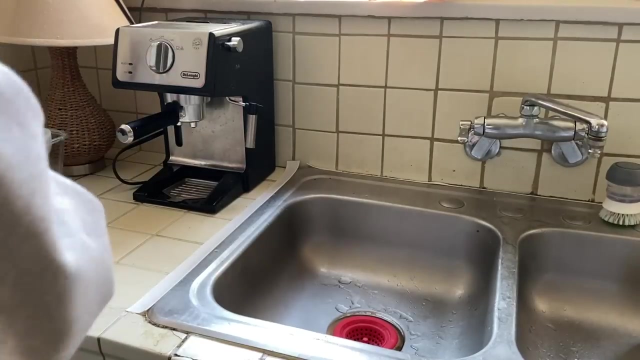 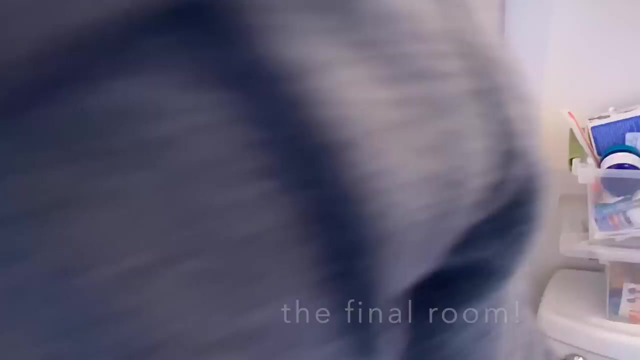 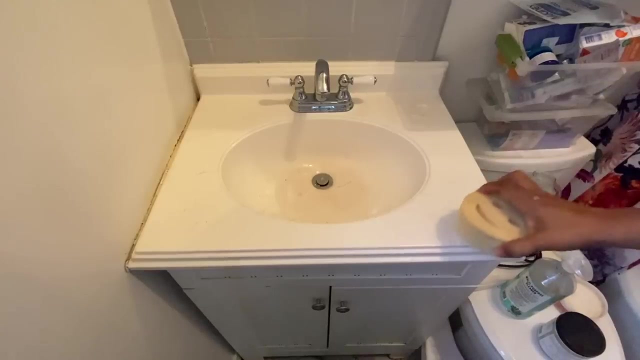 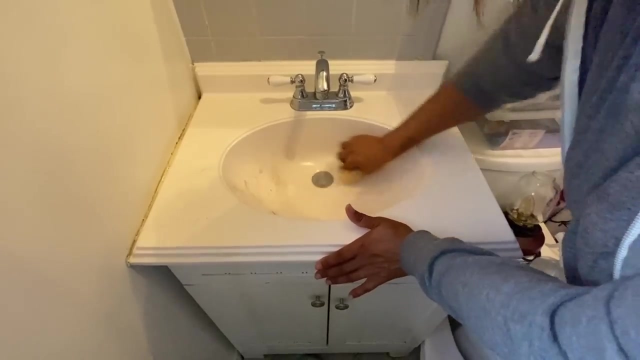 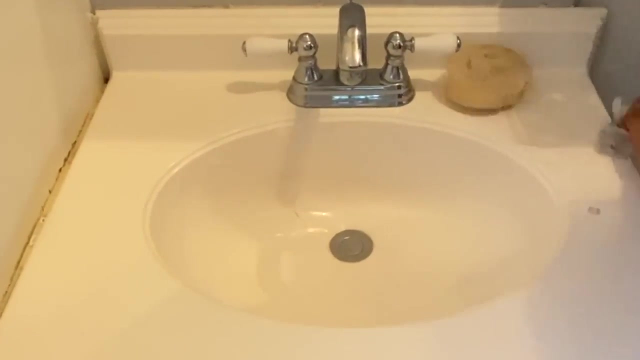 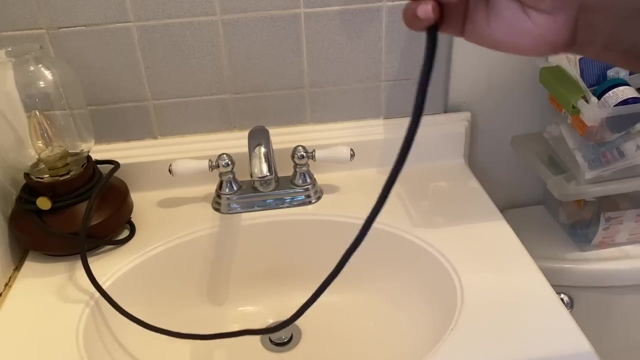 Oh, I even have my rollerball in here. It's great for all kinds of random things. I'm going to put this in the bathroom- my biomedic necklace- and I'm going to put this in the bathroom. I'm going to put this in the bathroom. 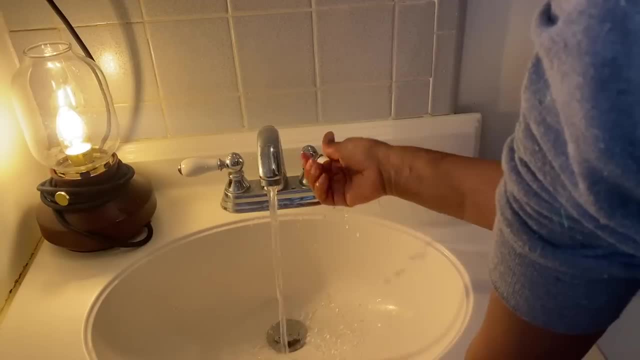 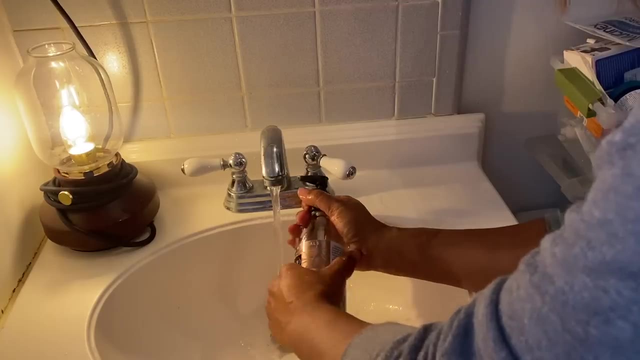 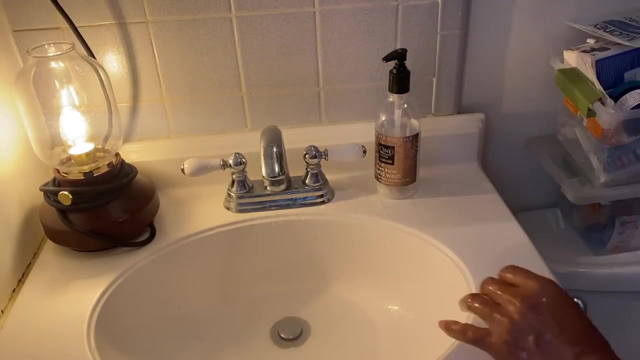 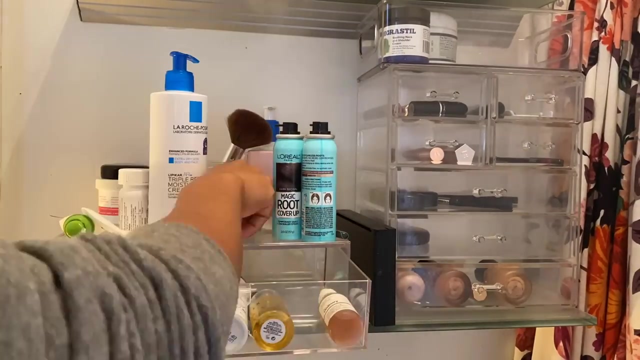 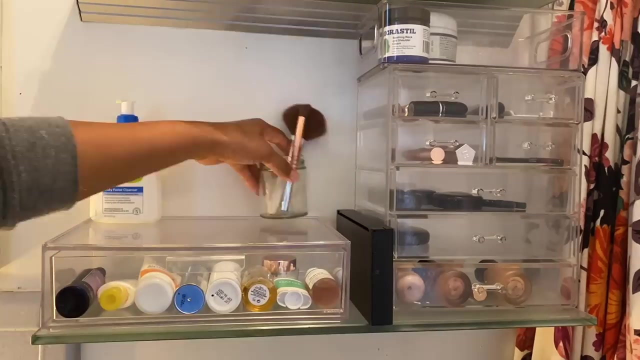 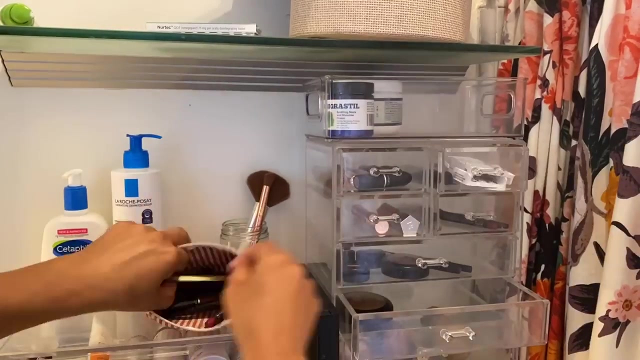 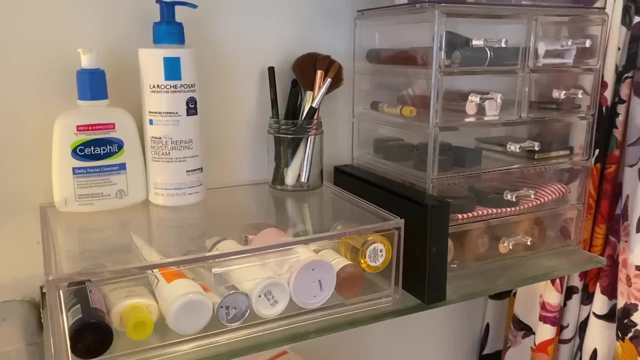 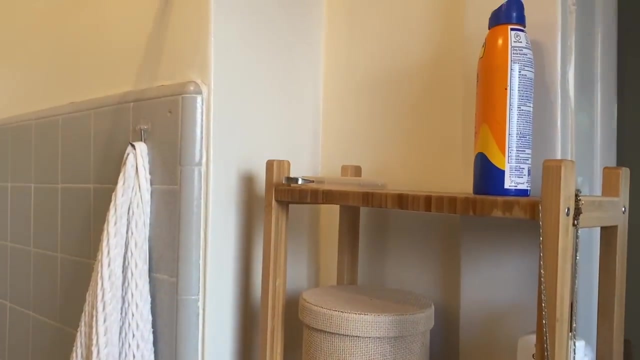 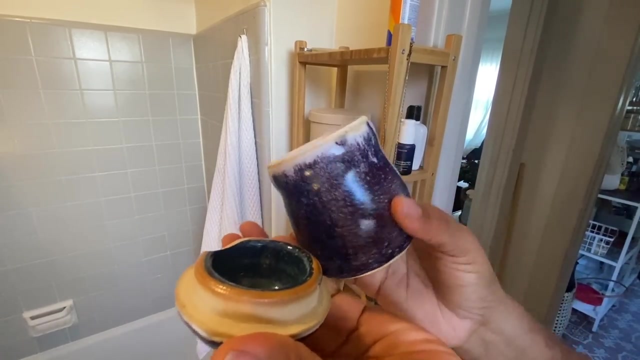 I'm going to put this in the bathroom. Much better, Much, much better. Let me work on this zone next. I love finding little jars like this. I found this at the thrift store. I'm going to put my coins in here. 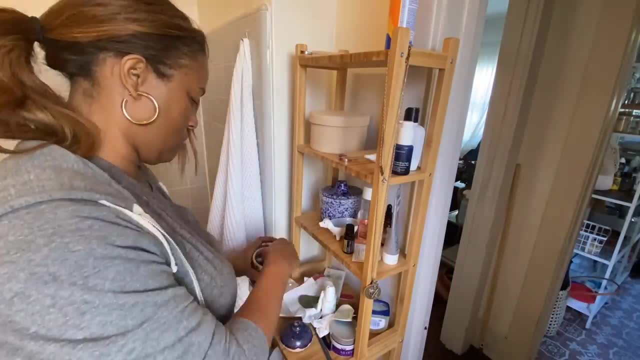 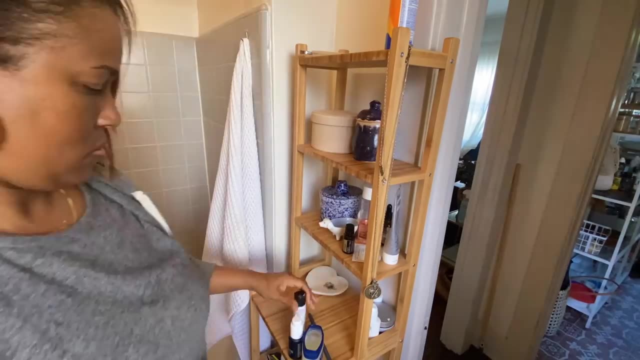 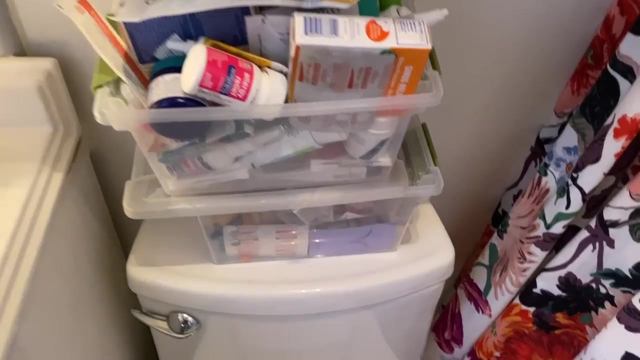 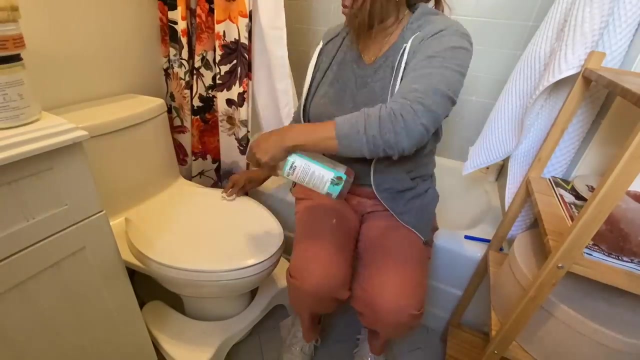 I'm going to put my contact lenses inside. Had this out because I was sick, so I'm going to move these under the sink. Okay, this looks good. This looks good. This looks good. I'll put this back. I'm going to the sink.